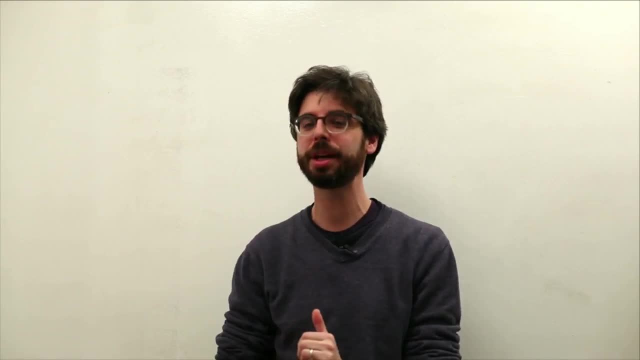 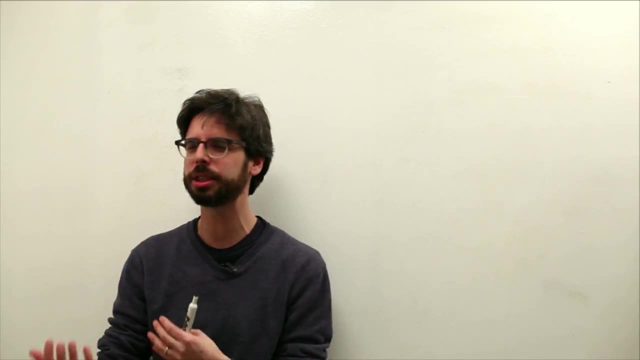 This is the third principle of object-oriented programming, and it's actually going to be something hopefully quite simple for us to understand. So we saw a hint of this. by the way, before We had this particle system, which managed particles. Then we made this square particle class. 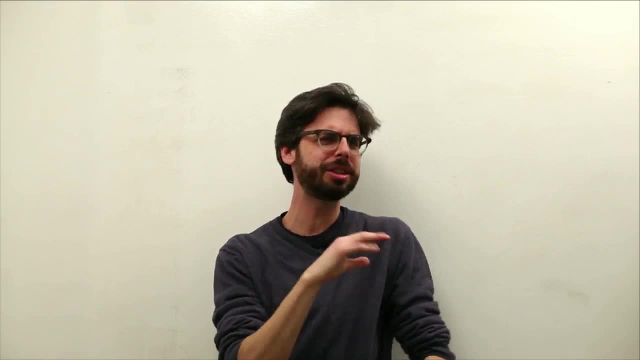 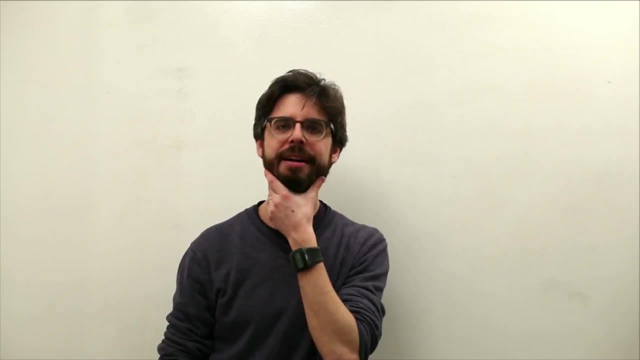 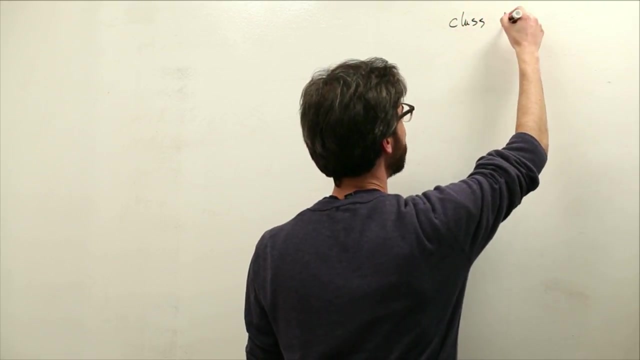 which was a child of particle, and we were able to put that in the particle system and everything just worked. How did that happen? Well, let's think of a similar scenario. Let's say we have an array, Okay. well, let's actually just say for a second: we have a class called animal. 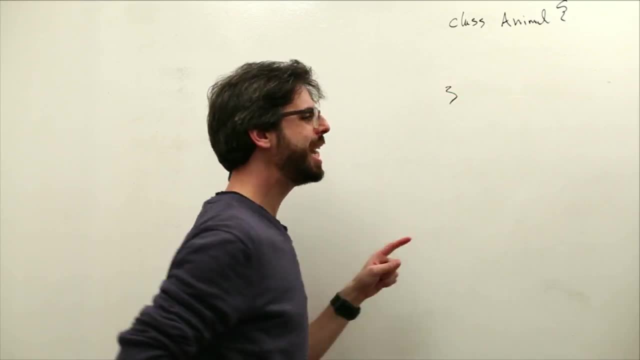 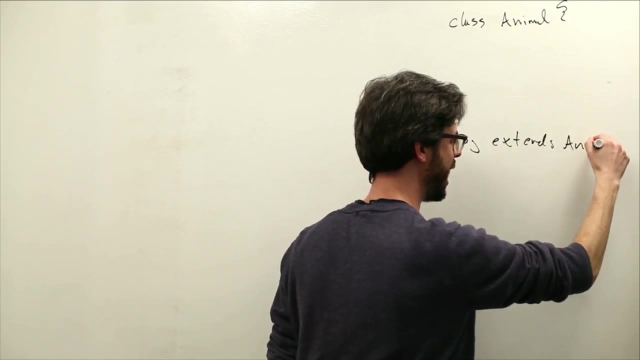 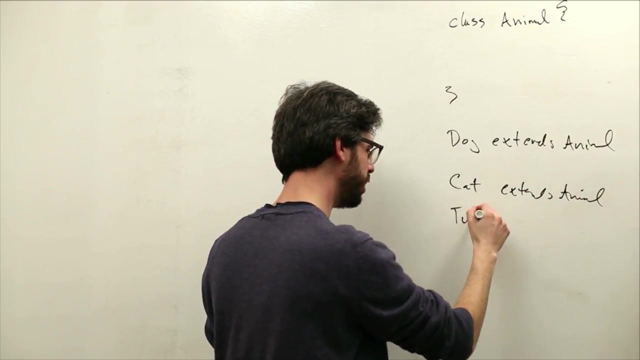 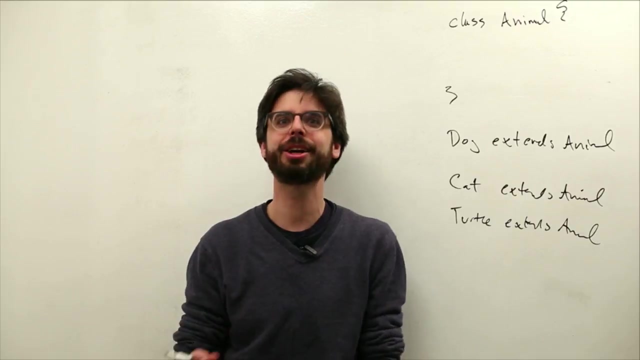 And let's say we have a class called dog And dog extends animal. And we have a class called cat And cat extends animal. And we have a class called turtle And turtle extends animal. Right, you can see where this is going. We could have this base animal class like our base particle. 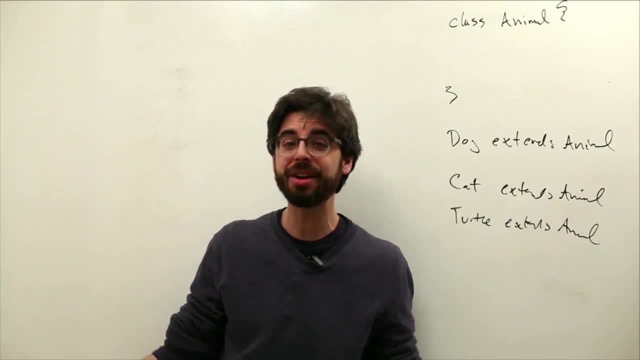 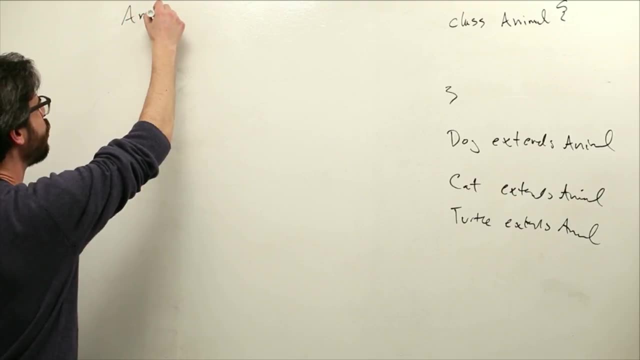 class and lots of subclasses that have all the basic functionality and data of an animal, but with their own customization. Now what we want to do is make an array In our particle system example. we're going to use array lists, But just for thinking it through right now, 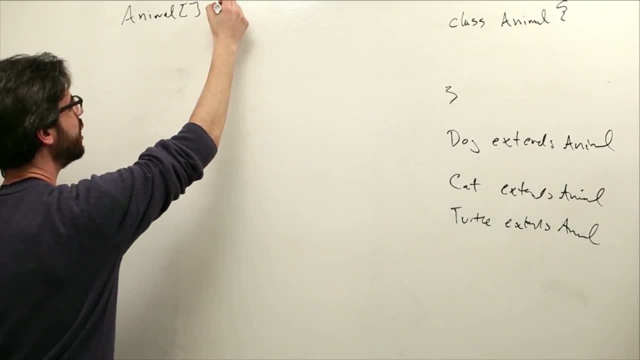 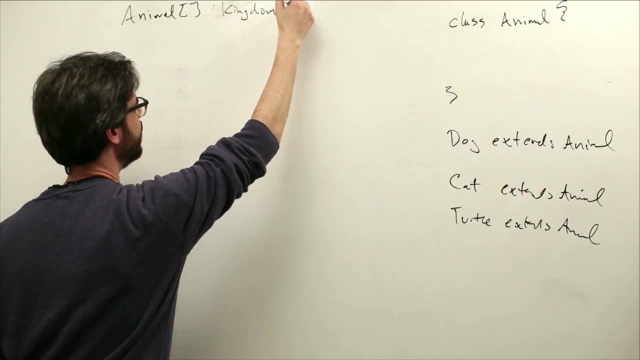 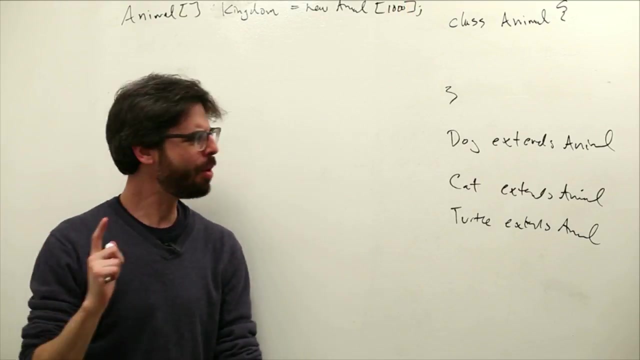 let's use a plain old array. We're going to make an animal array called kingdom Kingdom, which is a new animal array, And you know we're going to have a thousand animals in it. Okay, I want to put. 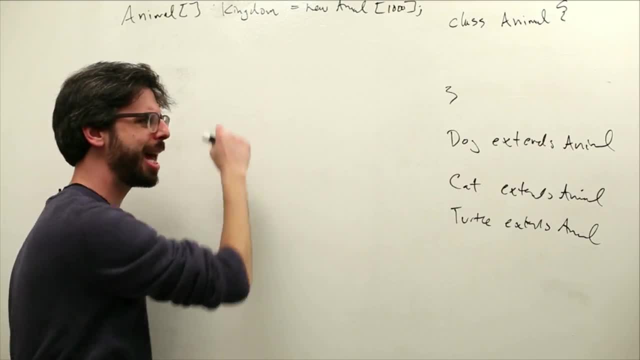 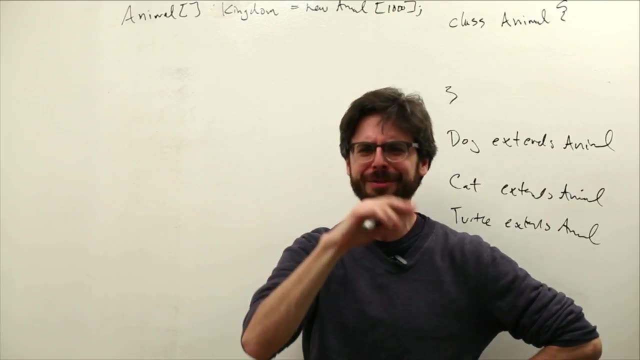 dogs and cats and turtles into that array. Can I do that? The answer, of course, is yes, Otherwise why would we be here? But just think back to. would that have been your first instinct. Maybe you would have said: I'm making a processing sketch and I'm going to have all these different objects on the screen. 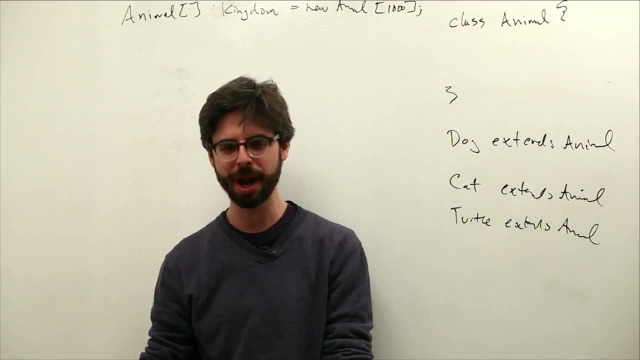 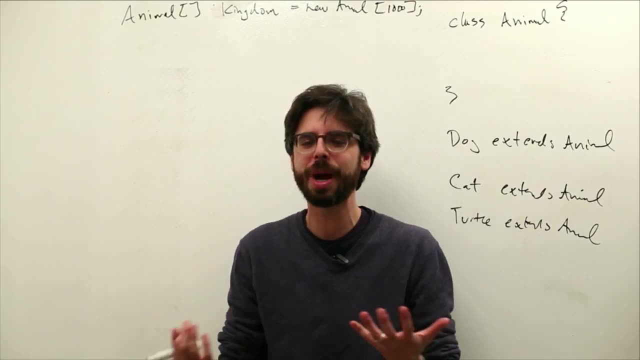 I need my dog array to keep track of all my dogs. I need my cat array to keep track of all my cats. I need my turtle array to keep track of all my turtles. This is going to get unwieldy pretty fast In some cases. you might want that, But the whole. 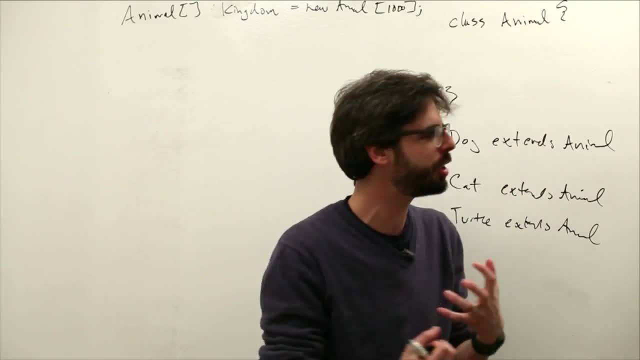 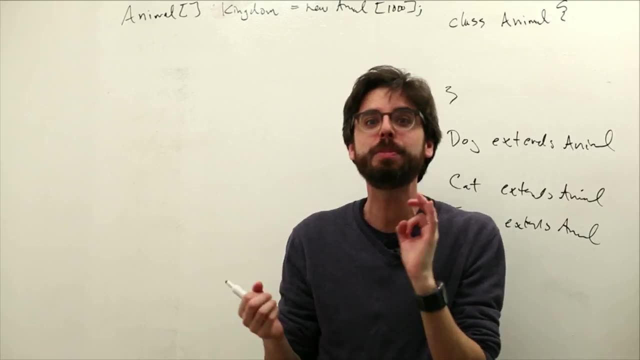 one of the reasons for doing this inheritance structure is it allows us to kind of collect all of these objects that have the same parents together and work with them together. This is polymorphism. This is going to. polymorphism is going to allow us to put all these different kinds 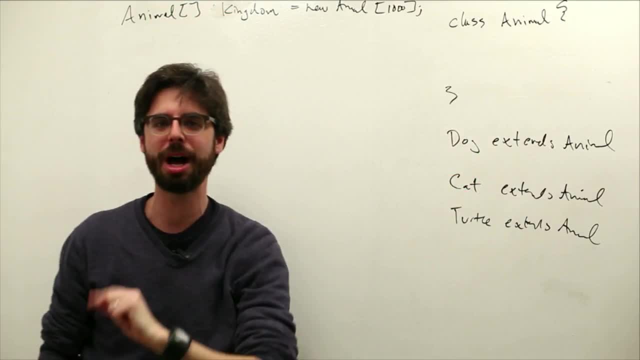 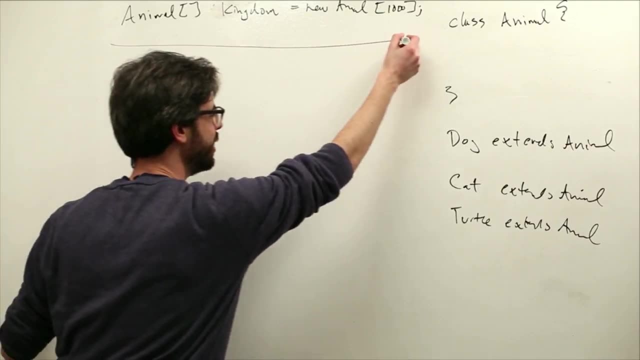 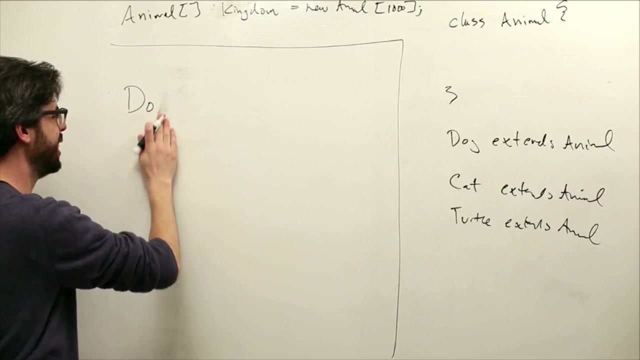 of animals into the same generic array of animal objects. Array of generic animal objects, I think, is what I meant to say. So let's look at two lines of code that I'm going to write out here. I'm going to say: dog, dog, dog rover equals new dog. Okay, this is something we should be very comfortable with. 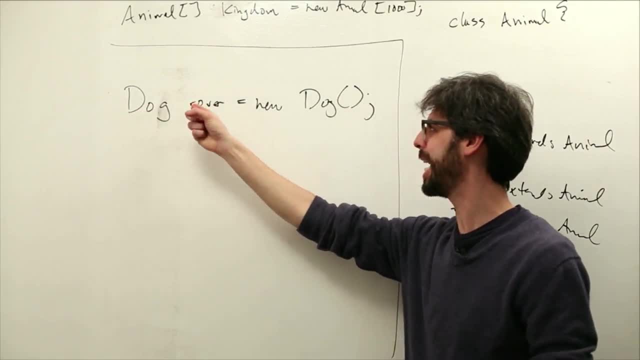 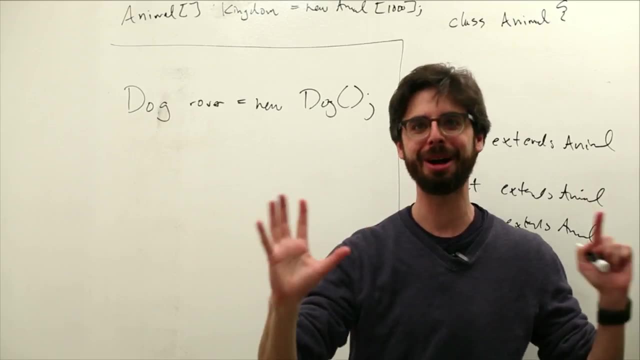 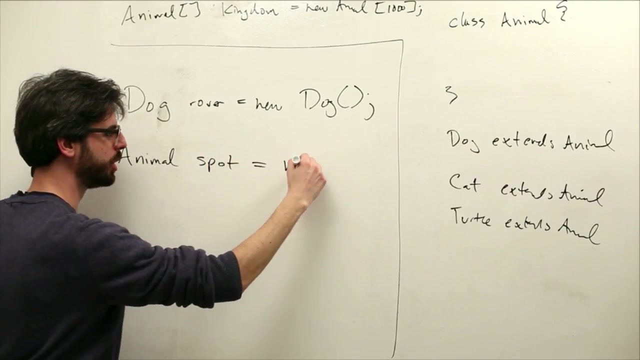 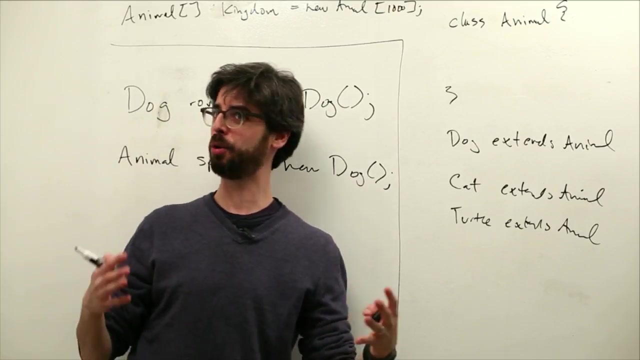 We're very comfortable saying: I have an object of type dog, its name is rover, it's a new dog object. Great, Here is polymorphism, something new that we're allowed to do. Animal spot equals new dog. This is polymorphism. What polymorphism? which means from the Greek? 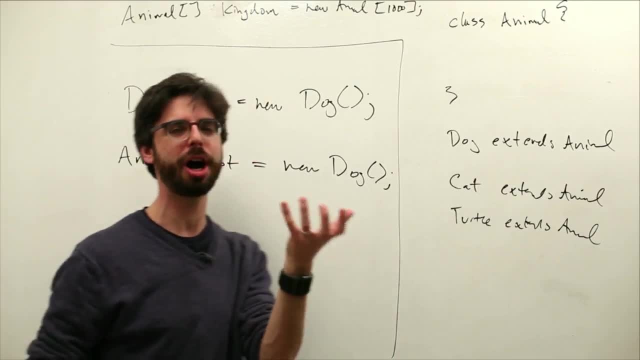 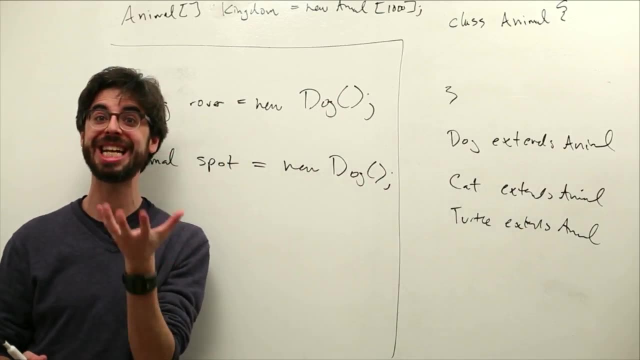 many forms. what it allows us to do is say: I have a dog object, And if it's convenient for me to think of it as a dog object, I'm happy to do so. If it's more convenient for me to think of it as an animal object, that's also allowed. I mean, it really truly is a. 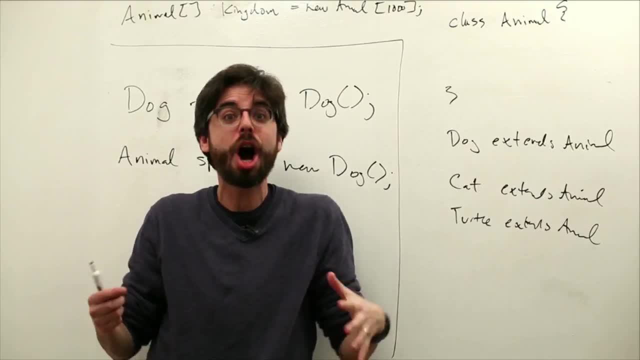 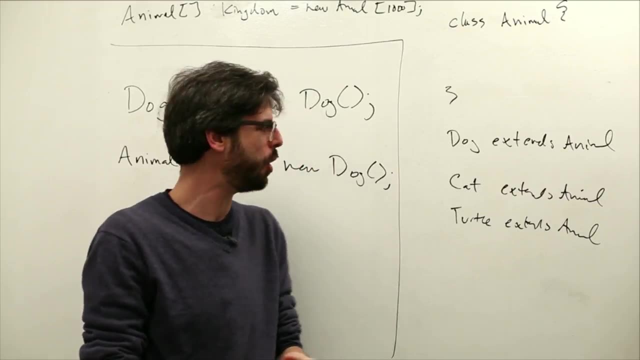 dog. A dog is a dog, is a dog is a dog, But we can talk about it as if it's an animal. because a dog is an animal, It's a child A class. a dog is made from a child class of animal. We can make an animal object which 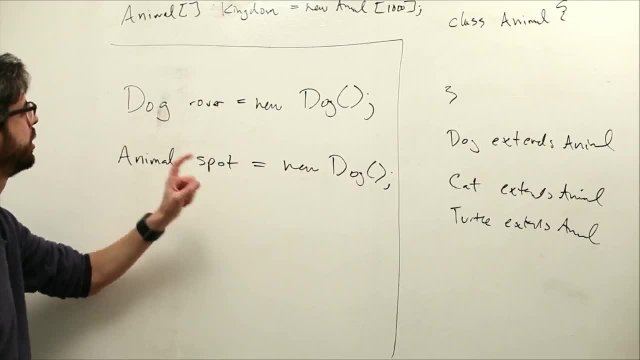 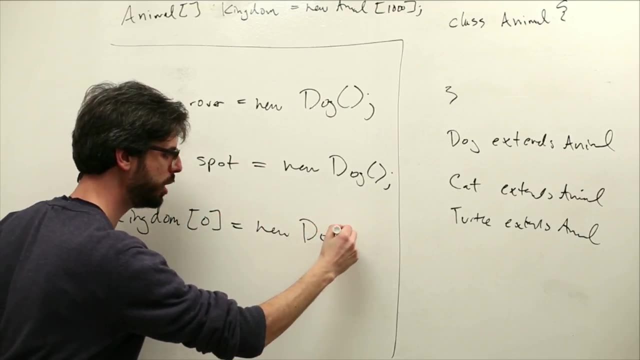 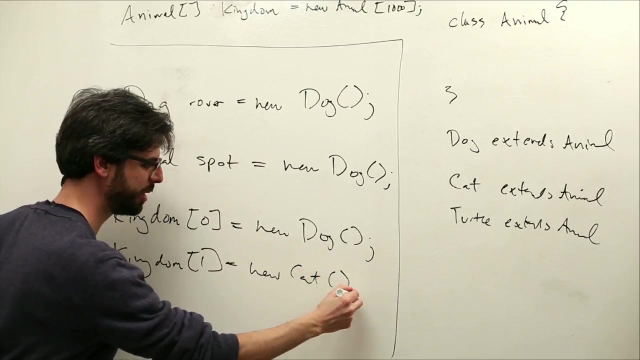 is specifically a dog. This is what allows us to put: kingdom index 0,, for example, could be a new dog. Kingdom index 1 could be a new cat. This is the magic of polymorphism. Kingdom is just a bunch of animals. A dog is an animal, A cat is an animal. 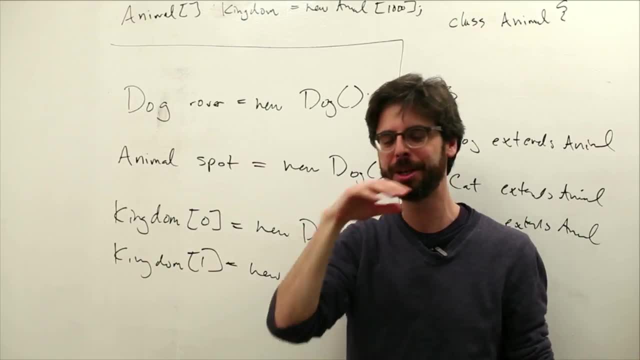 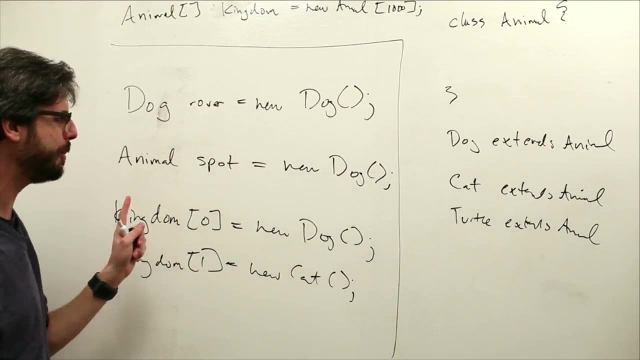 We can collect all these different kinds of classes into the same array. Great right. So hopefully this makes sense to you. but there's one little piece of this that I think would be worth mapping out: What happens when we loop through that array. And we know now. 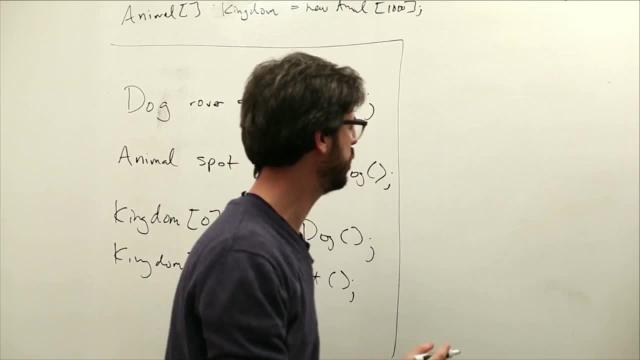 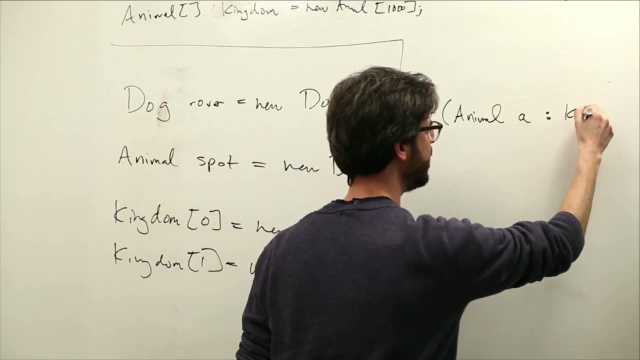 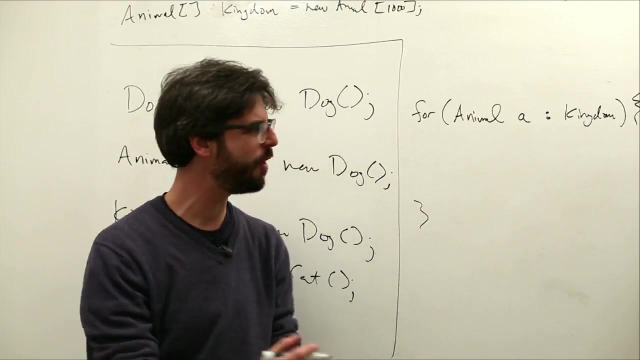 by the way that we have this new kind of loop that we can do. We can say: for every animal A in the kingdom array, we can say: for every animal A in the kingdom array. I could say: and what do our animals have? They had a sleep function and an eat function. 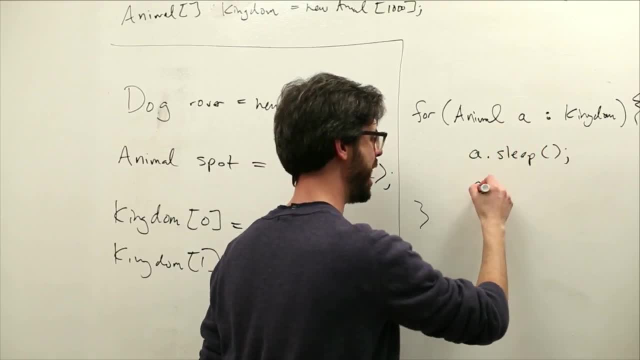 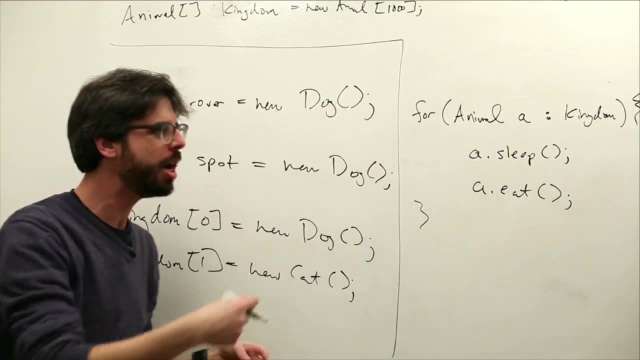 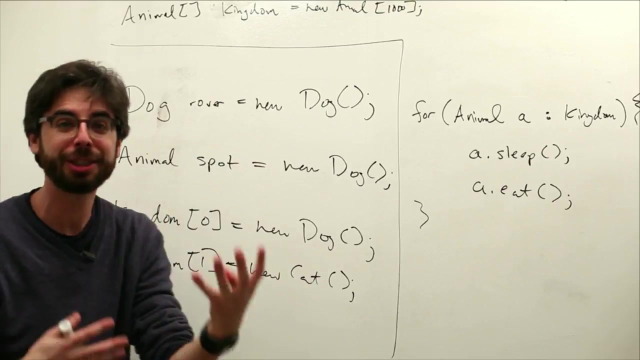 I could say: A dot sleep, A dot eat. So I could still loop through all of the animals and when it gets to each one I don't have to say: if it's a dog, sleep like a dog. If it's a cat, sleep like a cat. The magic of polymorphism and inheritance is it just knows. 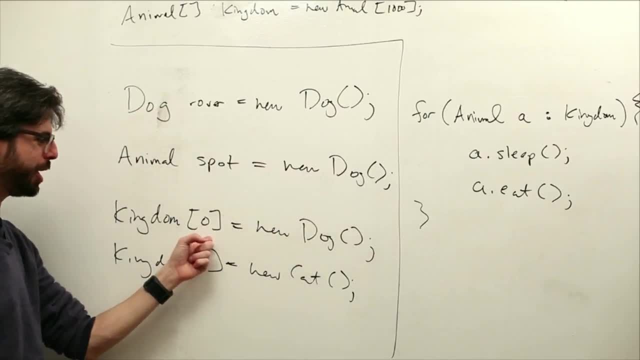 how to do it. It knows like. we made a dog and put it in the first spot, We made a cat and put it in the first spot. We're both animals, but a dog is a dog is a dog is a dog. When it gets to sleep it's. 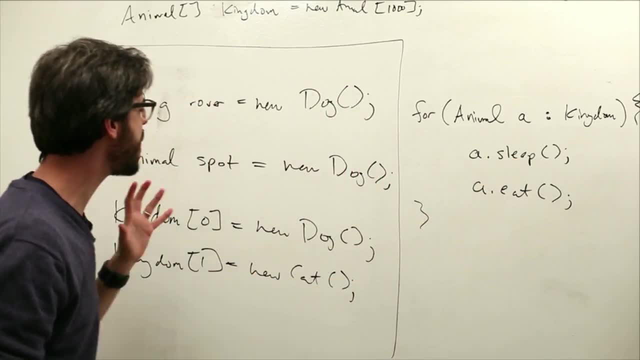 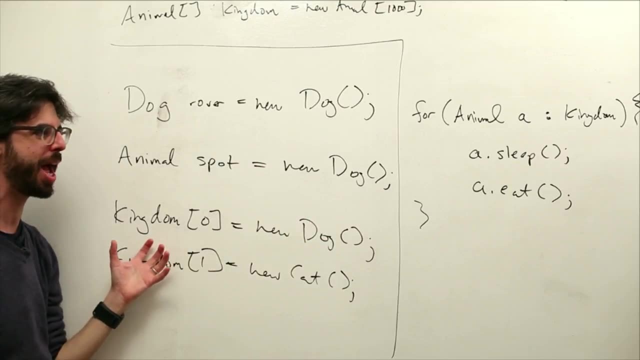 going to sleep like a dog. When it gets to eat, it's going to eat like a dog. So this is very powerful. We can have an array of generic animals. We can put specific kinds of animals in that array, We can loop through all of them and we don't have to keep track. 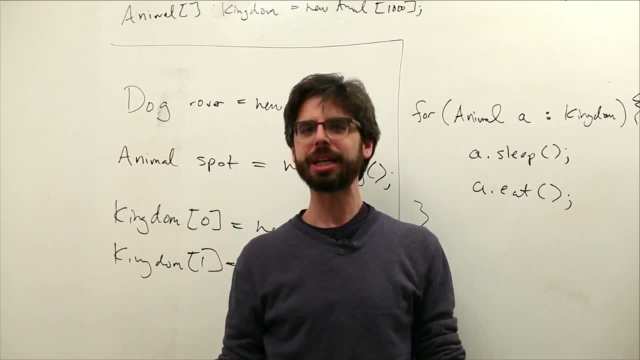 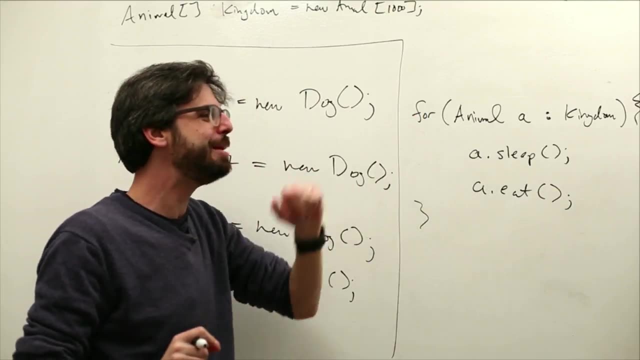 of which one is which Java slash processing. slash the computer, the little people inside the computer pulling in all the switches and buttons in there. it keeps track of all that. for us, This is incredibly powerful. It's going to allow us to make a particle system full of. 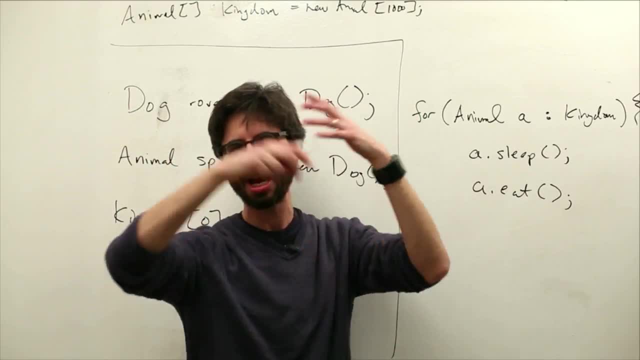 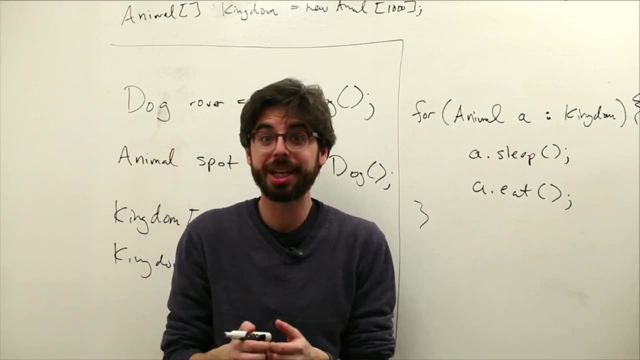 particles- square particles, spinning particles, star particles, rainbow particles- And we don't have to keep track of what's what. We can just put whatever we want in it. We can say they're all particles and the program is going to keep track of that for us. 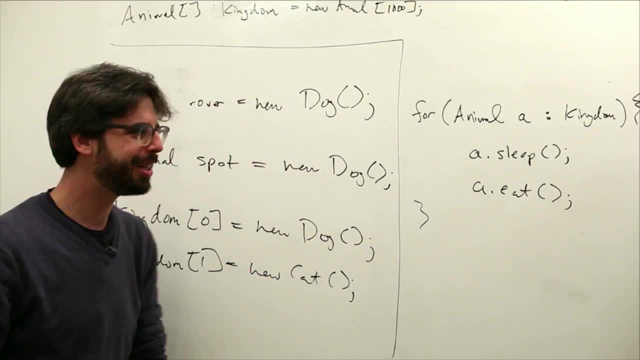 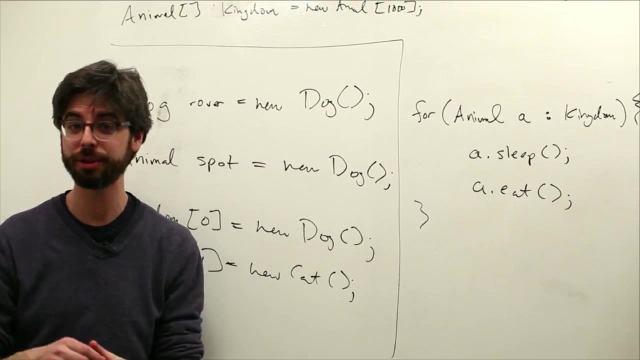 OK, I'm hoping this makes sense to you. If not, we will remedy that situation somehow. But so let's actually go now back to our particle system example. I forgot to turn the timer on, so I don't know how long this has been, but I think it's a good amount of time. So 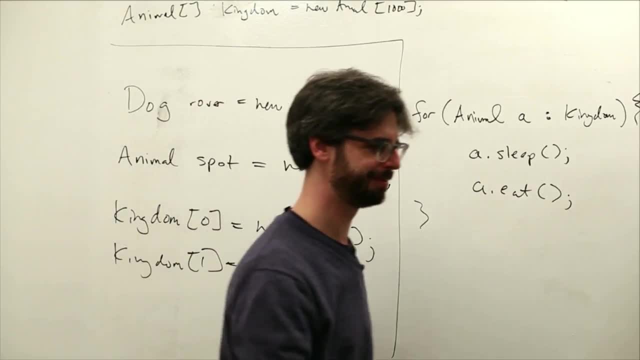 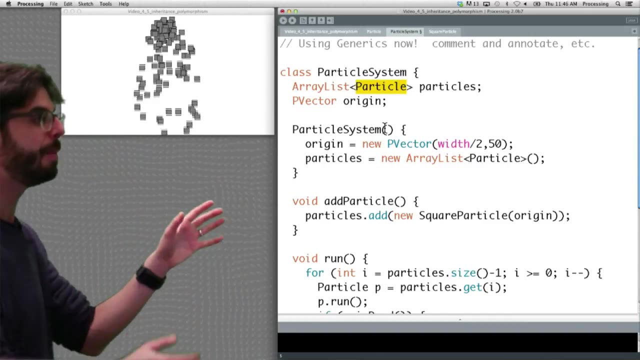 let's go back to our particle system example and let's see polymorphism in action. OK, so, if you remember, we actually have polymorphism in action right here, because we are putting square particles in the ArrayList, but the ArrayList type is a generic particle And 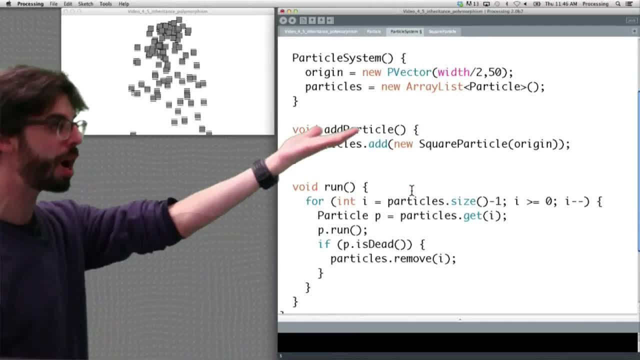 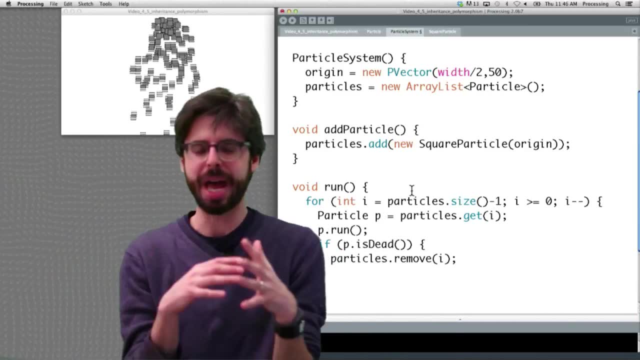 we can see here, we're treating a square particle as a square particle when we want to make it, but as a regular particle when we're accessing it, because this is us looking at it in different forms. So this is polymorphism in action. 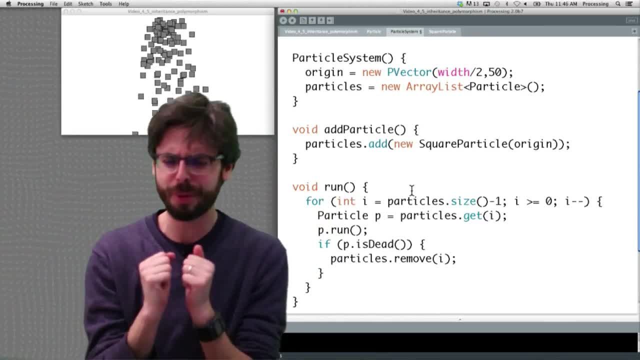 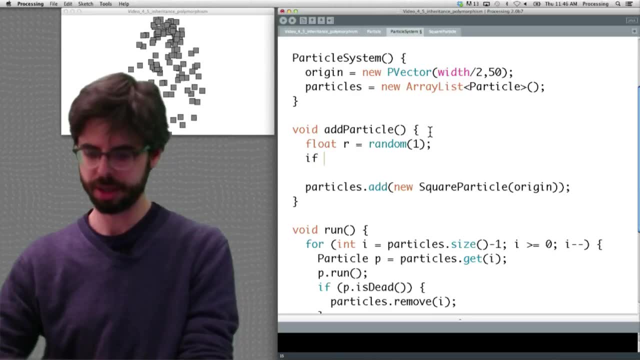 But let's really prove to ourselves that this is working- and I'm going to add just a little piece of functionality here. I'm going to pick a random number between 0 and 1, and I'm going to say: if that random number is less than 0.4,, there's a 40% chance of